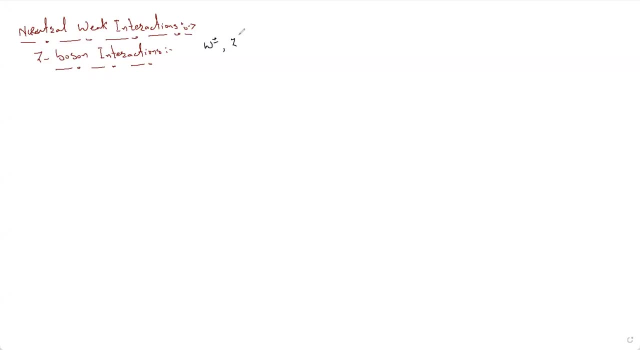 particle. in terms of the weak interactions, either W plus minus or Z zero. In the last case, we were discussing about the weak interactions that are mediated by W plus minus And we call those interactions as the current-current interactions. Now, today, we are going to talk. 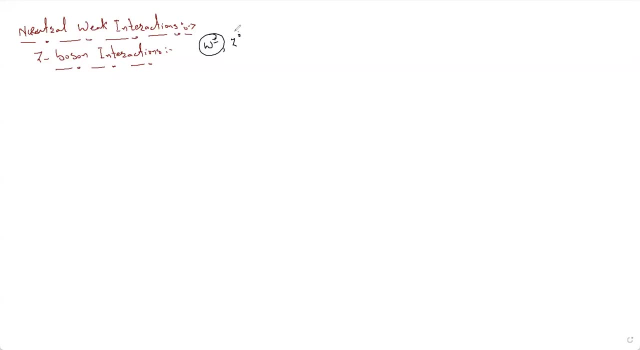 about or discuss about the neutral-current interactions, That is, the weak interactions, where we have the mediating particle as the Z zero boson, Or simply we call this as a Z boson. Now, if you remember, in the last time, we see that as the exchange of this. 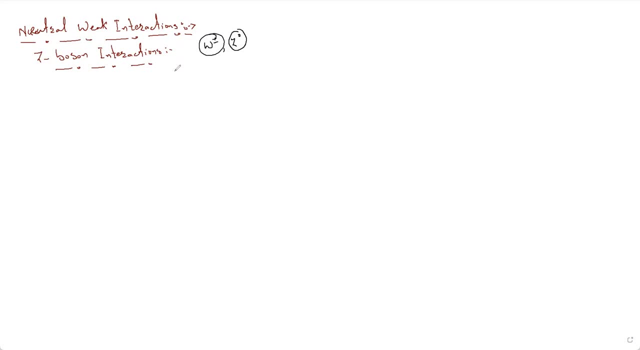 W plus minus happens. the flavor is changing. What I mean by the flavor is changing. that means the up-cork. we see that the up-cork goes down-cork, That is, this U-cork will couple to W plus minus and it will change to the 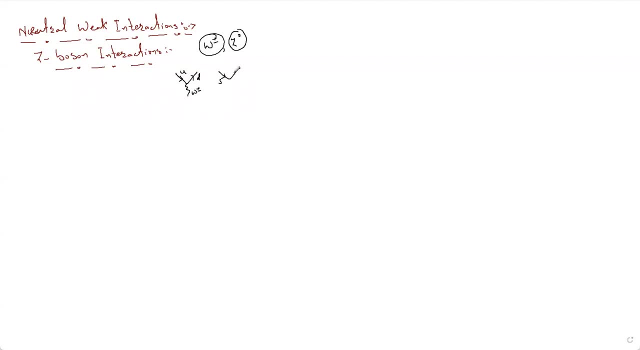 down-cork. Similarly, the string will go to the charm-cork and the top-cork will go to the bottom-cork, with the coupling of this W plus minus Right. This is the case when we were discussing of the current-current interactions. Now, besides that, these weak 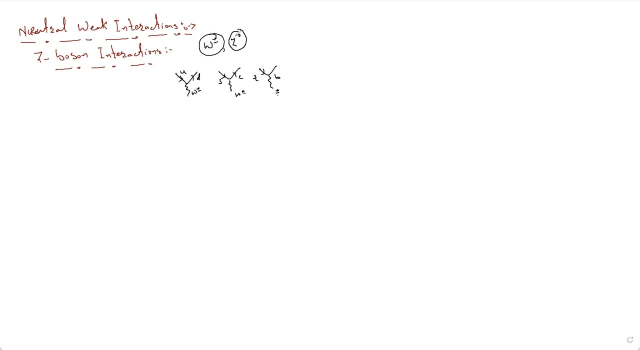 interactions are mediated by the neutral-current interactions. Now, besides that, these weak interactions are mediated by the neutral-current interactions. Now, besides that, these weak interactions are also mediated by these Z zero bosons. Okay, So we call them as neutral-gauge. 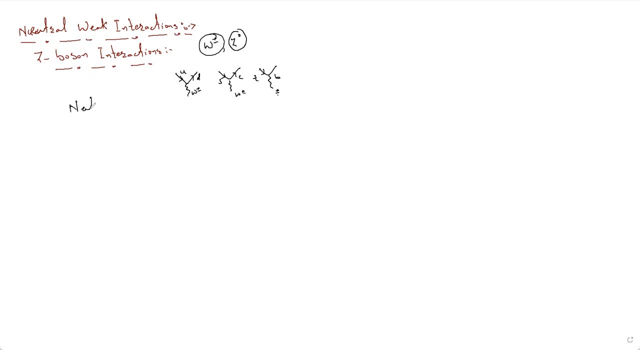 bosons, Neutral-gauge bosons, Neutral-gauge bosons, Or simply we call this as a Z zero. Okay, Now, this Z zero. like we see that in this current-current interaction, this W plus minus couples to corcus as well as the leptons. 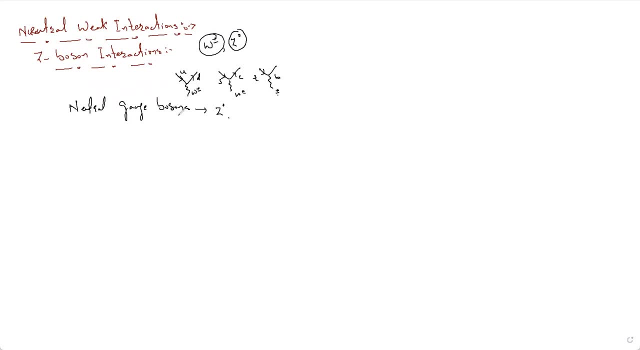 Now this W, the Z zero boson, also coupled to corcus as well as the leptons. but it does not change the flavor. What I mean by it does not change the flavor means here up-cork goes to down-cork. So once it couples with the W plus minus it up will change its flavor. 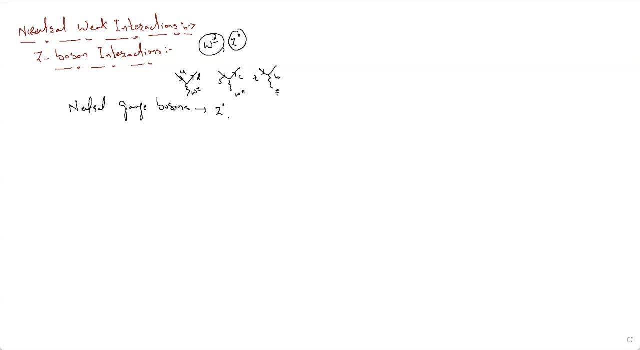 to go to the down-cork. Similarly, the string will go to charm and so on, But the Z zero, in this case in Z zero boson. this will couple to the both corcus as well as the leptons, but the flavor. 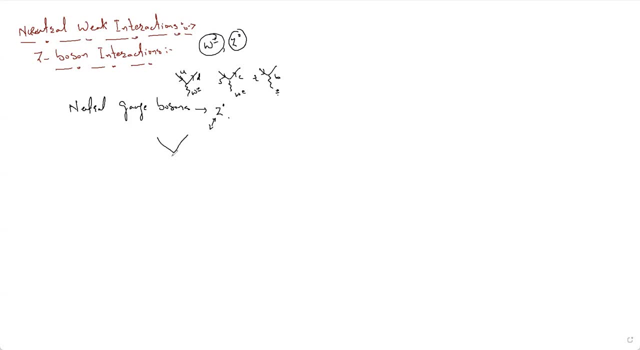 the flavor is not changed, So let me represent it by some diagram. So here, if this is, F stands for some cork or a lepton, or simply some fermion, because corks and leptons are fermions. So the same, this fermion goes out, which comes in Again, it does not change. 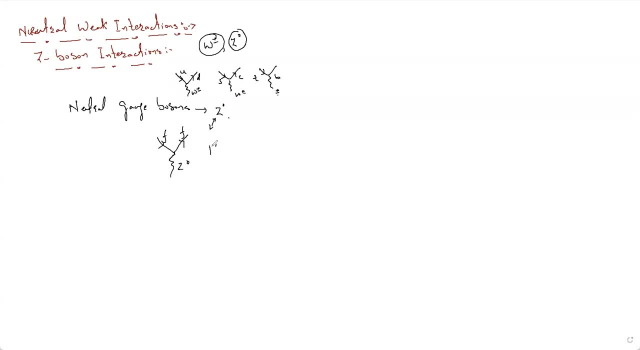 the flavor once it interacts with. So there is no change in flavor in case of this Z, zero exchange, No change of flavor, Whereas we see in the previous case the flavor is not changing its weight because that is the difference between the two polymers. So now, if we go, 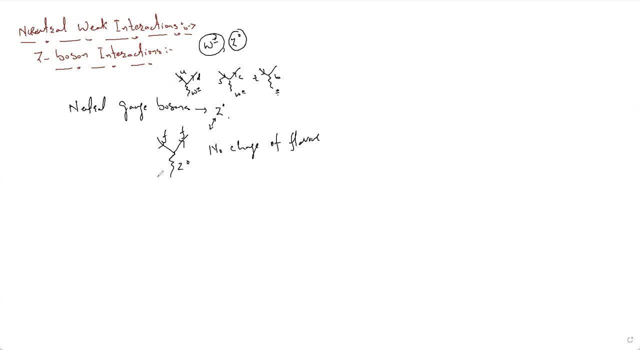 to the next one and the first one. it is all the same. So now we go to the next one and the first one. So the two leptons are very similar, So they are all the same. Now makes: 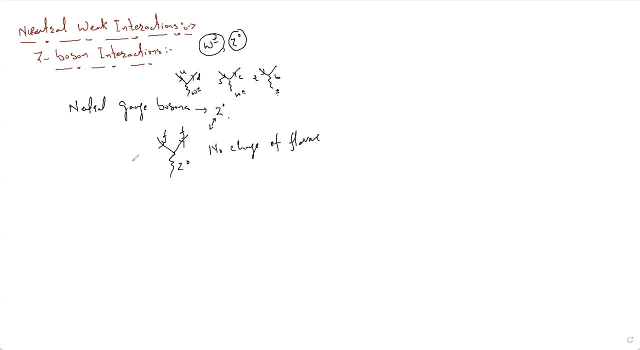 it a little bit easier to assimilate. We have to make sure that that the two levels are being changing while we are talking about the corks or the leptons. So if we look at this particular interaction, since the plumber does not change, So we can say that this inflections is very much similar to that of the photons, because we know that when some particle will interact with a photon, when the mediating part is, like in electromagnet case, the particular remains are like, for example, the scattering of an electron. 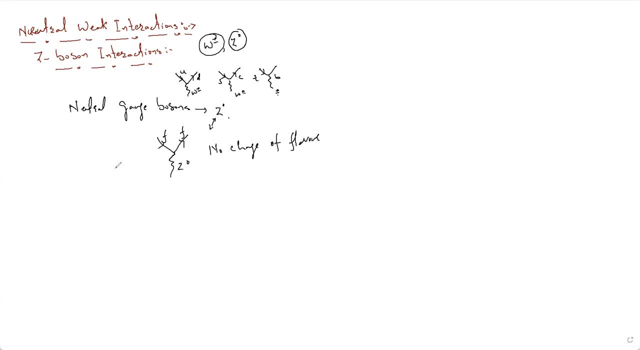 electron comes, electron goes and there is an exchange of uh. it couples with a photon because the photon is in this mediating quarter in case of the electromagnetic interaction. then what makes this z zero different from that photon exchange? okay, so there are actually two important properties which make it different from that photon interaction. the first one is that this z 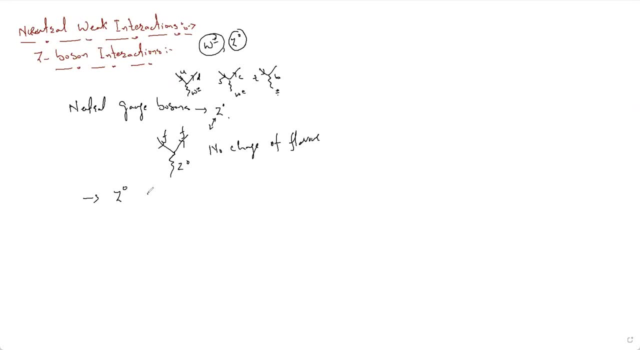 zero, johan. it couples to the neutrinos. this z zero couples to neutrinos and you know that neutrinos are massless particles, neutrinos, whereas the photons do not. so that is the main difference. photons do not right, because the neutrinos also have zero electric charge. they are electrically neutral. 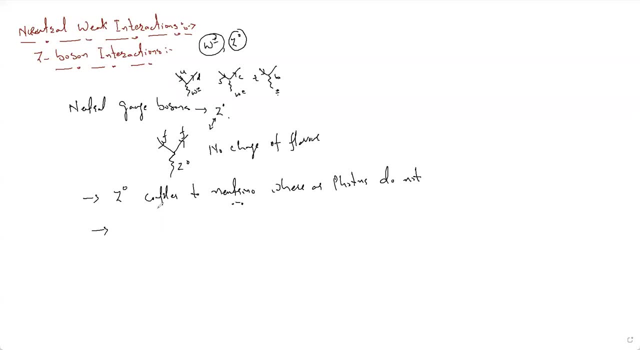 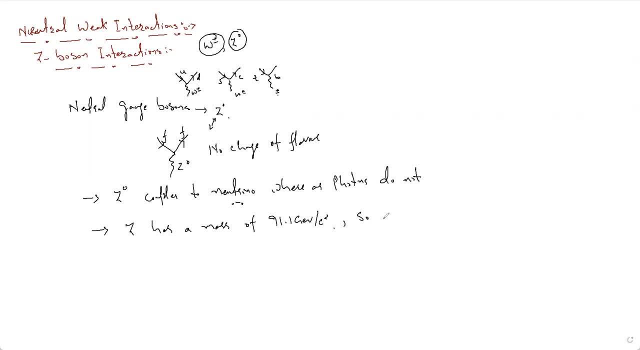 square. so that is why. so this is the reason that the this, these interactions are short range. weak interactions are short range. so the interactions are short range because of the mass of this mediating particle. short range- okay, try to understand it in a very simple way. say that the weak interactions are mediated by two particles mediating. 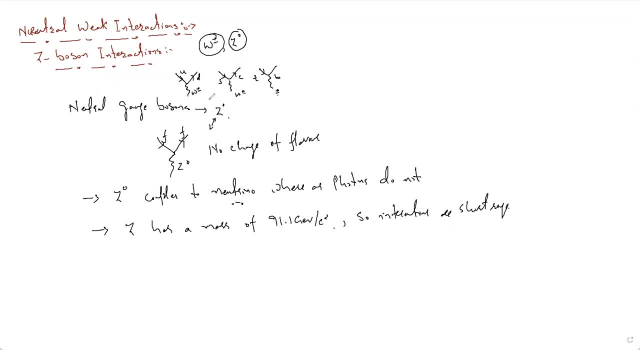 quanta one is w plus minus, whereas the interactions where the mediating quanta is w plus minus, we call them as a current, current interaction and those weak interactions where the mediating quanta is your z boson's at gauge neutral gauge boson, we call those interactions or neutral weak. 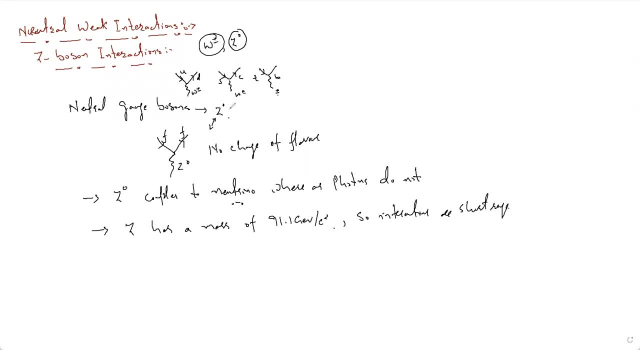 interactions or z boson interactions. right now, in the previous case, we see that the flavor of the cox changes once it's coupled with w plus minus like these in cases, whereas in of this z boson interaction, the flavor does not change again if the same particle comes out, which 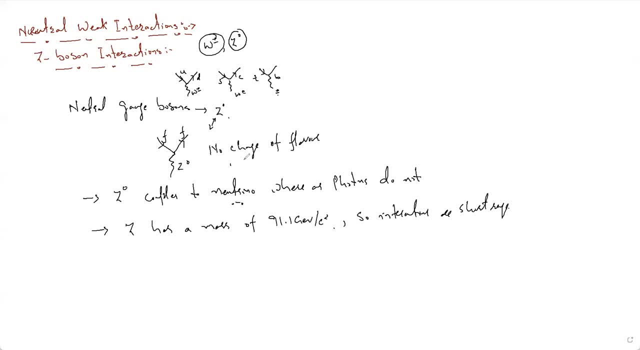 comes, goes out, which comes in. there is no change in the flavor when there isn't, when there, when this, uh, fermion or some quark or electron, couples with z zero. so these interactions, we can say that, since the flavor does not change, so we say that they are similar to the photon interaction. some 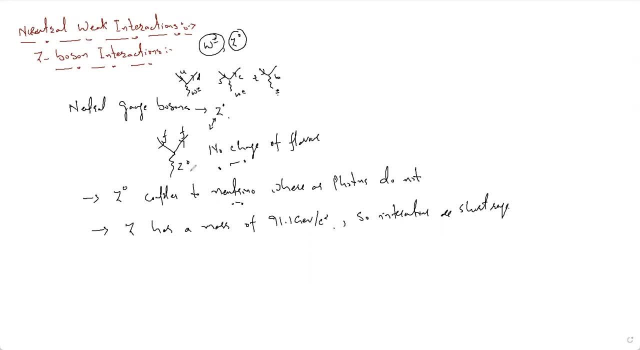 electromagnetic interaction. but what makes it different from that electromagnetic interaction? one thing is that zero will couple to neutrinos, whereas the photons do not couple to the neutrinos, and the second is that it has a mass of this, whereas you know the mass of this photon, it's actually a massless particle, very small mass, less, almost zero mass. so 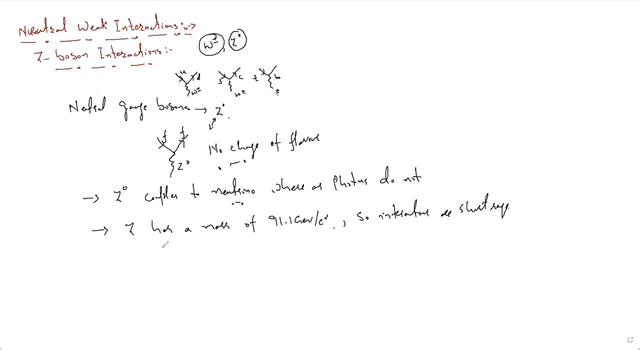 nevertheless, uh, i will say: in any process where there can be a photon exchange, there can also be a z. so in any process where there is a photon exchange, there can also be a z zero exchange. what i mean by this? for example, i will consider an electron, electron positron scattering, for example. 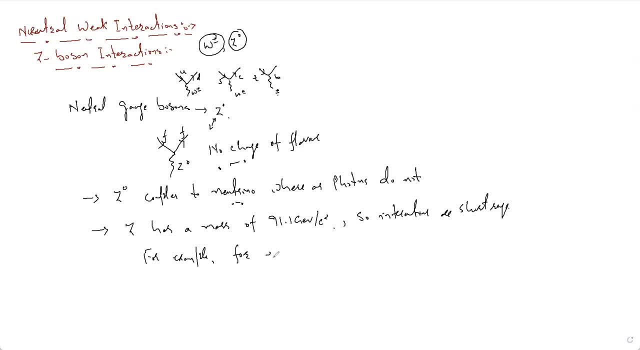 i consider an for electron positron. this is an anti-particle of an electron scattering into a pair of final state particles. into a pair of final state particles, what actually happens? the electron will annihilate a positron as a result. so they are massive particles and it's conversion of mass into the energy. so as a result, we will get 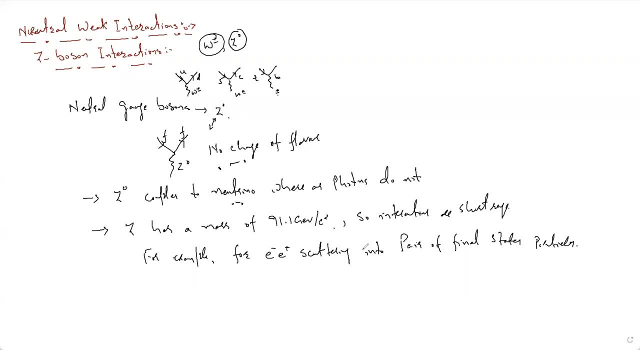 some energy, and that energy is being released in the form of photons. so let me make this with the help of this diagram. so i'm making two diagrams where, in the one case, i will show the photon exchange and then there is a zero exchange. okay, so let me write it like this: 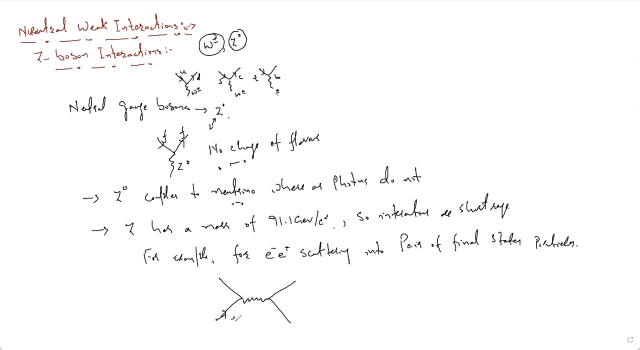 okay, fine. so, as i said, we have some electron and this is some positron. we are representing it outgoing in the fanman diagram. as a result, we will get two: this photons gamma, so there is actually a photon exchange here. gamma: we are actually representing it as 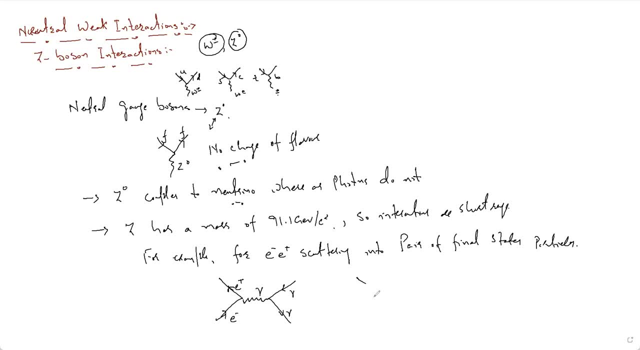 a photon exchange, also the same process. i can also represent it by like this: here we again have the two gammas coming out, and here we have an electron and this is a. this is a positron here, but the mediating chorda here is a z zero. 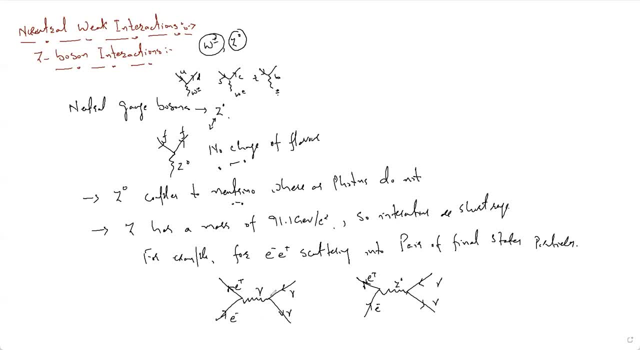 z boson. now, obviously we know that when there is some exchange process, there is some propagator involved, like we see in the case of the current current interaction. now, what is the propagating operator? the propagating water? in case of an electromagnetic, this photon exchange, the 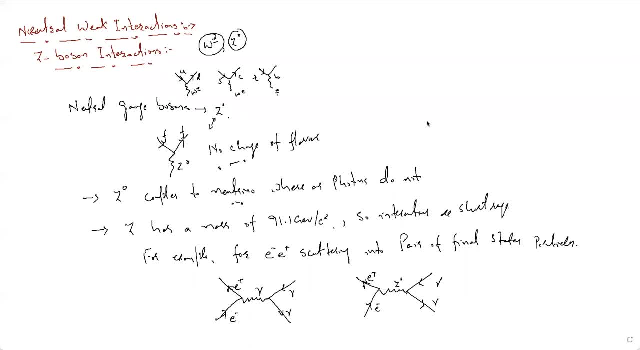 propagator here. let me write it here: the photon exchange. the photon exchange has a propagator, propagator 1 by s. now, what is this? s s is the centra mascara of the central mass energy, because centric center of mass energy will be presented by 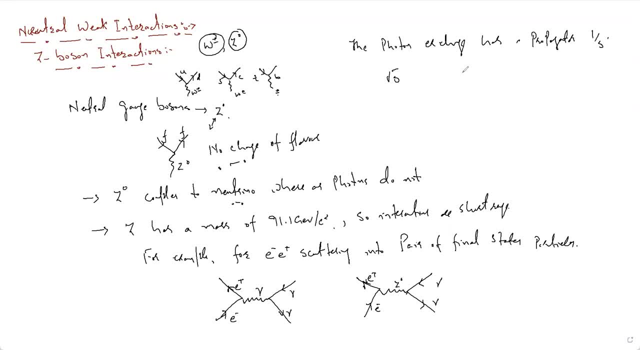 under root s. so s here will be the care of the center of mass energy. so where s is actually the center of mass energy? center of mass energy. we have discussed what i mean by the center of mass energy, whereas the z exchange has a propagator of this particular this is. this is for this particular case and for 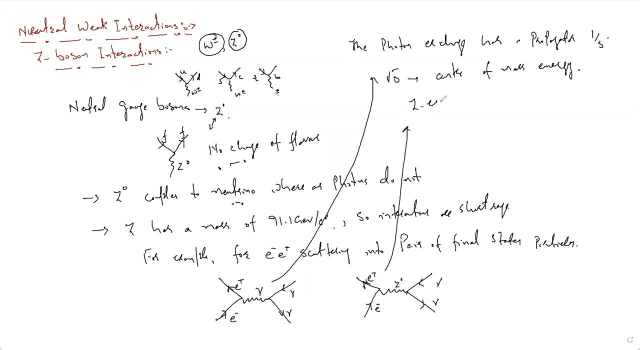 this particular case where we have a z exchange, the z exchange has a propagator. propagator: it's given by 1, by s minus m z squared c 4, m z squared c 4. okay, this is the propagator in this case. and in the case of a photon exchange, we simply have an photon exchange, uh, this. 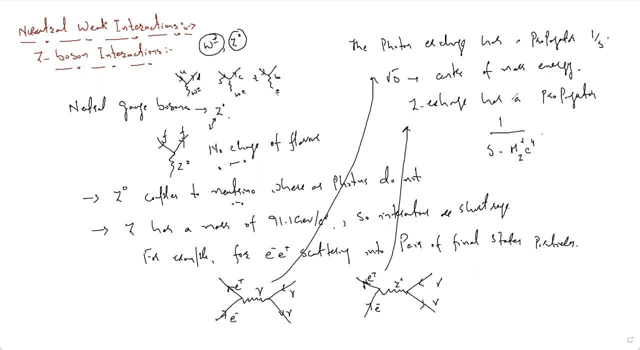 propagator of 1 by s, that is the center of mass energy. now i am discussing here two different cases. now for relatively low center of mass energy, that means where this under root s is very less, is very less. so for less center of mass energies, what will happen? this center of? 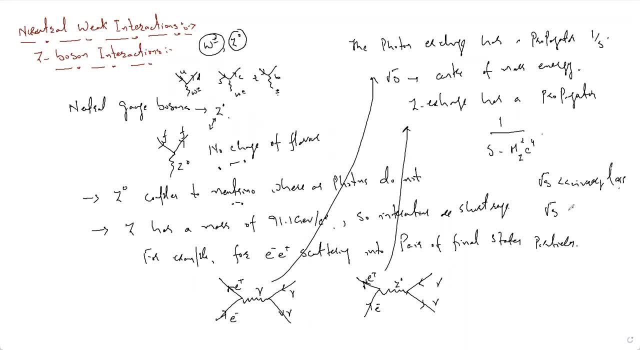 mass energy. what i mean by less? that means this center of mass energy root of s should be very much less than this mz c squared and in the mass of the z zero boson. so it's like that means, for example, we know that the mz c square is around your 91 or 92 gv, so that means the center of. 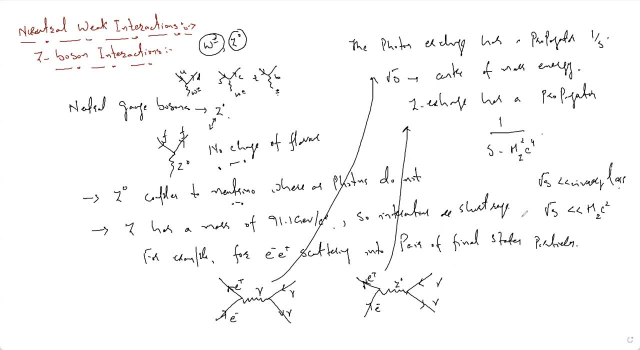 mass energy is very less. it will be around some 1 gv or 2 gv. so if i talk about the one gb or 2 gb, that will be considered as a less as compared to the rest mass of the z, the z boson. so in that particular case the z exchange process contributes least, so that exchange process 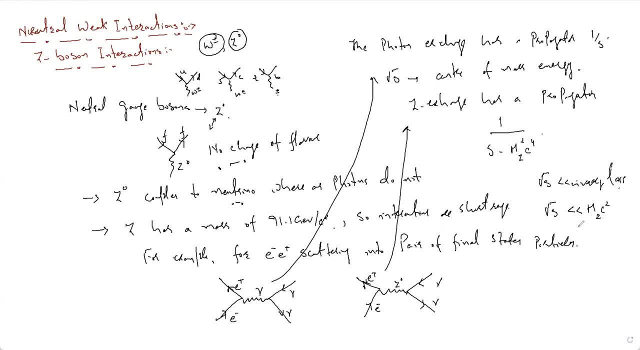 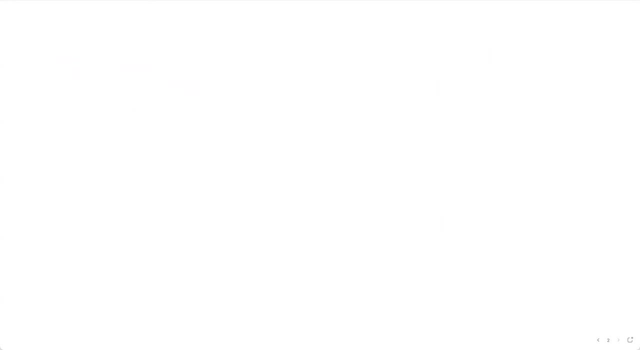 it will contribute least what i mean. so if it contributes this, it can be neglected. it can be neglected. let me go to the next page. okay, so this, this can be that exchange process contributes and can be neglected. however, as the scent this s grows. however, as this under root s grows. under root s grows means when the center of mass energy is. 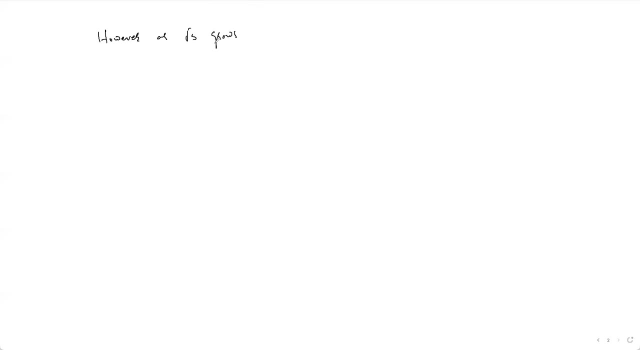 very high, so such growth size that it will become comparable or greater than this mz c square any this under root of s will become comparable or or greater than greater than this mz c square any rest mass of this z boson. both these diagrams are equally equivalent. which two diagrams are equally equivalent? 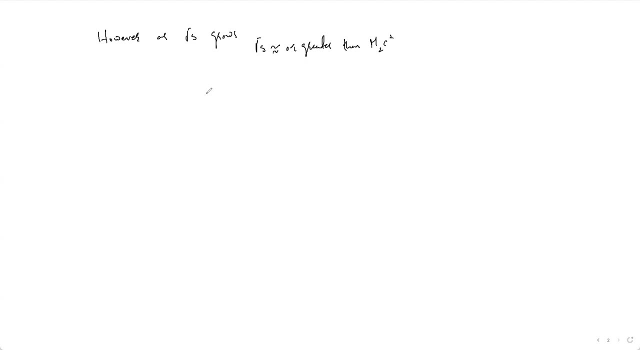 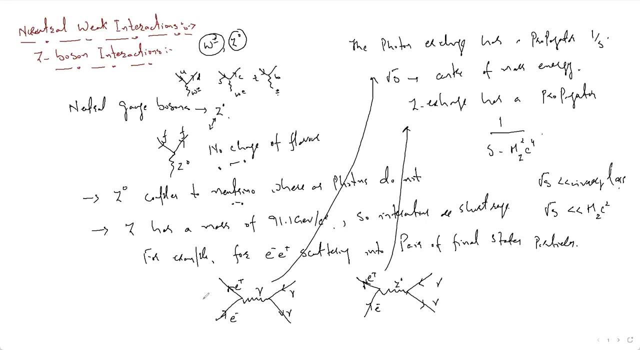 let me write, let me make the diagram here first. so like, for example: okay, both these diagrams are equally equivalent. that means these two diagrams, this diagram and this diagram. so when this is the case, this equivalent means when the center of mass energy is comparable, or i can say it's, it's greater than the rest mass of the zero boson. these diagrams are: 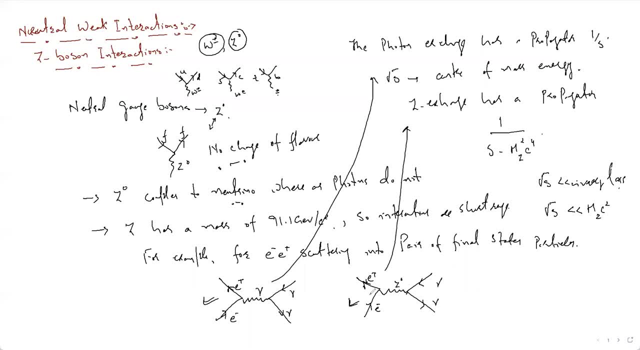 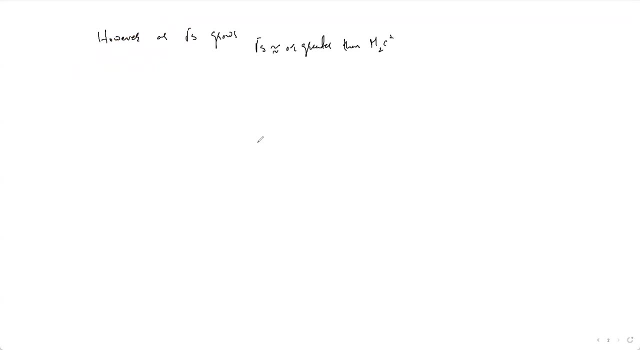 equally valid otherwise, for example, when the center of mass energy is very less, the mz c square can be neglected. and it can it. it contributes least and can be neglected. fine, okay, now there is another thing, uh, about this z and photon. so this z and photon also coupled to both w plus minus. 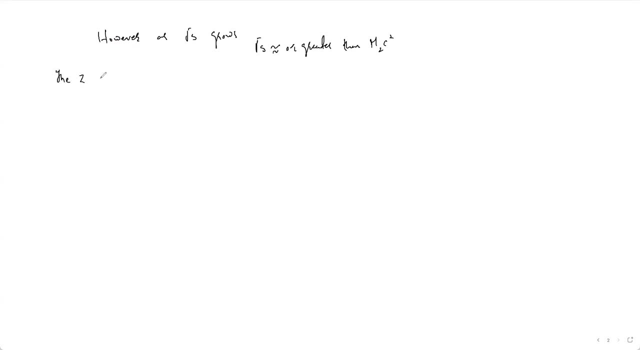 let me write in here: the z and photon can also coupled to w plus minus, like how it will couple to w plus minus, like in the first case we have. if this is a z, it will couple to this. sorry, like this and this: if is z, it will couple to w plus and w minus. so 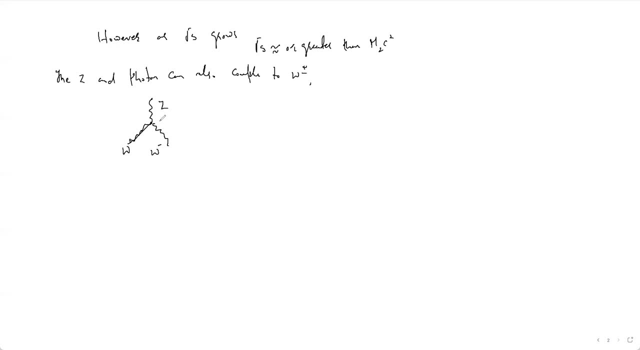 if this is w plus and w minus, what it means? it will couple to this. this z boson can go to w plus and w minus, also in case of a photon. if i have a photon, then i have a process like this: this is a photon, it will couple to w plus and w minus. okay, what is the authenticity of these two? 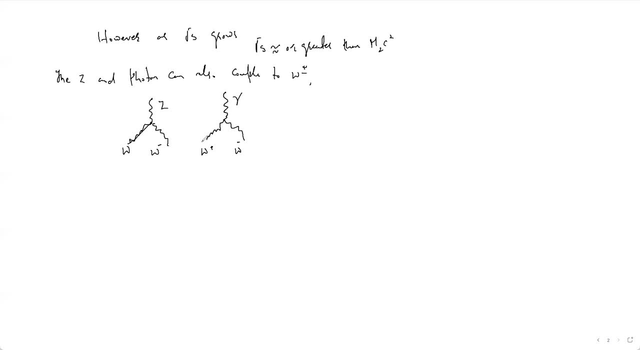 processes. actually, these couplings were confirmed experimentally at an at cern. so these couplings, this z couples to w plus and w minus, and this photon coupling to w plus and minus, these couplings were confirmed experimentally, experimentally. and this large electron proton collider. 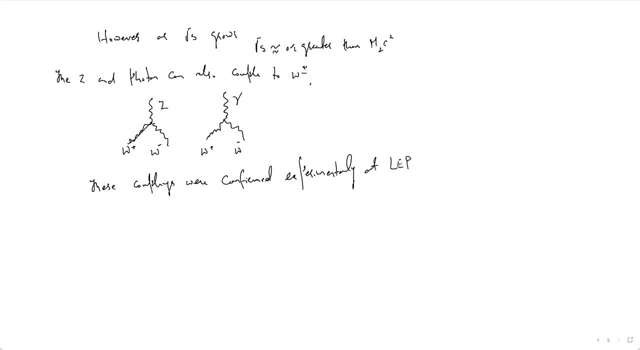 these are actually two. one is large electron proton collider. then there is the same, uh, another, this experimental facility that is called lep2. the lep1 is meant for some other processes, but there's an another experimenter setup which we call as lap second. so this is an experiment. 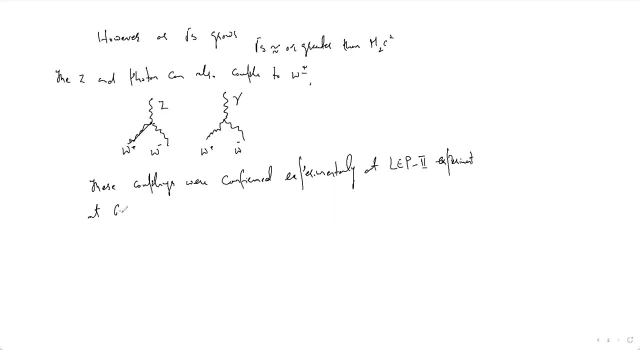 experiment at genema, this cern. so you know why, certainly us. and what is the properties of the, what are the different things we can do at the? certainly, like we had, large hadron collider is there, and so other experiments. we have discussed it about it in your last, in the last unit. okay, 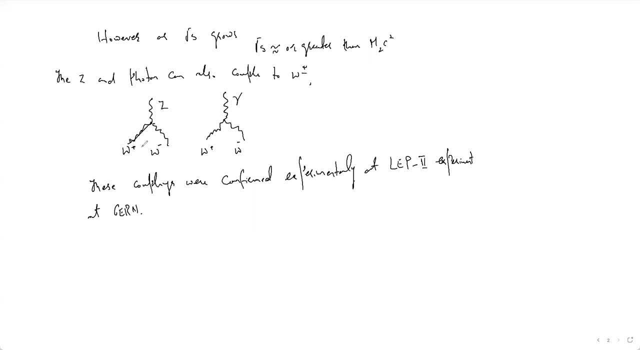 so, ah, these couplings, so this w coupling to w is the amount we have. so the co-alignment at the moment is in the fifth column. so this W-ad, So this W coupling to W plus and W minus, and photon coupling to W minus and W minus. 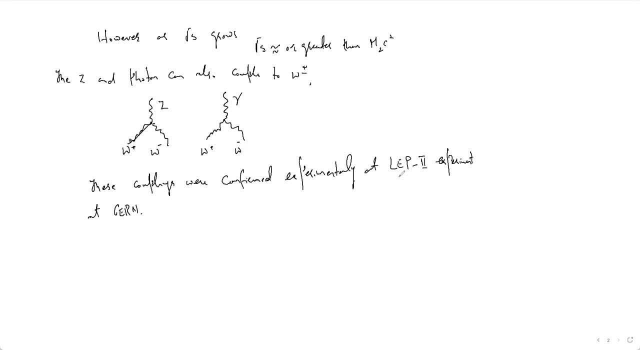 these actually were confirmed experimentally at this particular experiment, LEP Large Electron Proton Collider, which is called at CERN. What happened there? Actually, they just collide, accelerate these electrons and positrons to sufficient energies, and you know how the collision actually happens. so they actually made this from here an electron. 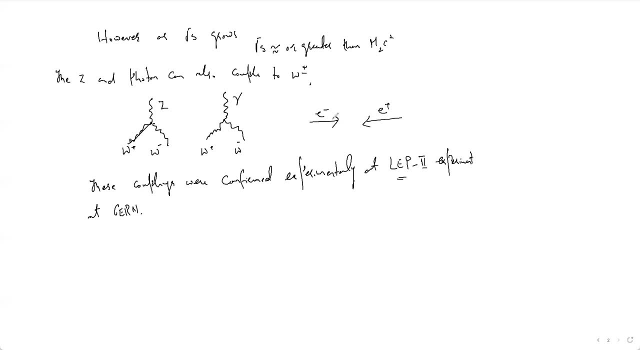 has come from here and a positron has come from here. they allow them to accelerate to sufficiently high energies to so, when they will interact, they will produce a W plus and W minus in the final state. So, for example, if this is an initial state, in the final state W plus and W minus were. 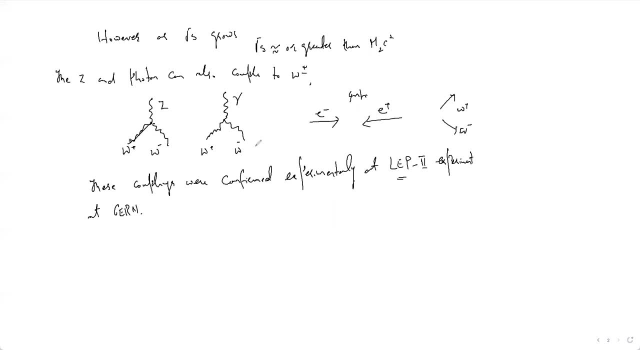 being produced in this particular interaction. So they confirmed with these couplings, with the help of this experiment, how they did that experiment. they actually allow the electron and the positron to collide at sufficiently high energies. As a result, in the final state particles by W plus and W minus. these two particles 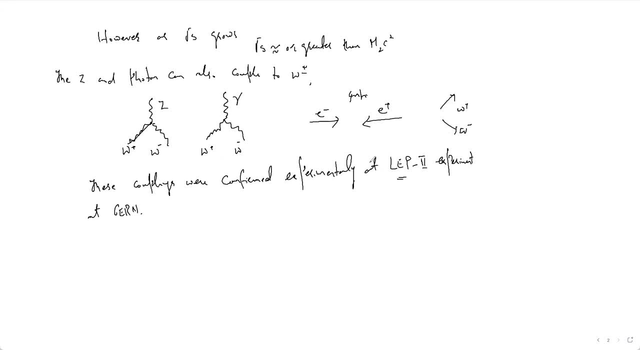 okay, because they are bosons and they were being observed in the final state. Okay now, from the coupling of this W plus to the electron and neutrino. so I will just represent it by the Feynman diagram. So the Feynman diagram showed the coupling of this W plus to electron and neutrino. 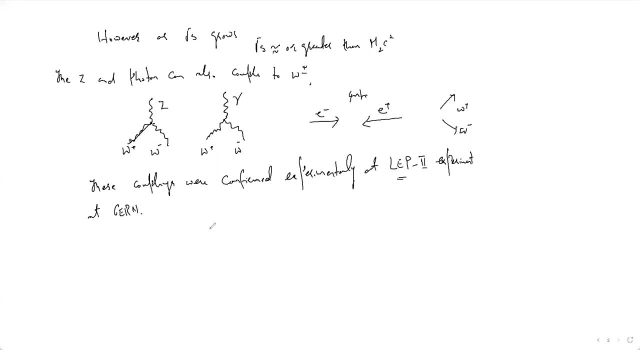 So let me just show you how it actually happens. okay, In the Feynman diagram, This is like this: okay, So here we have an electron coming in and this is in positron. okay, This is because they are coming in the opposite directions. that's why we are actually representing. 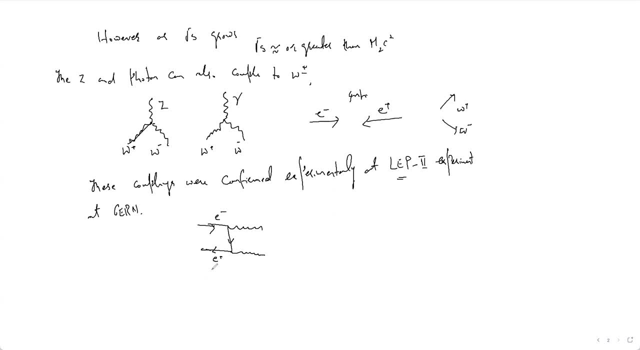 the Feynman diagram in this positron, the entire particle. we always show it with the outward arrow. Okay, this is some W minus and this is W plus minus. So this is the opposite direction. This is the opposite direction. So this process can be represented. this is a photon here. 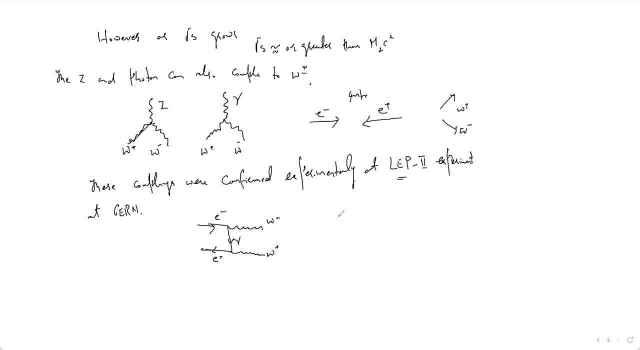 So we say that this W plus minus will, this electron positron will produce a final state particles. however, this Z and the photon also have coupling to W plus minus. So this is electron and positron will just collide and they will result in the production of a W plus and W minus. 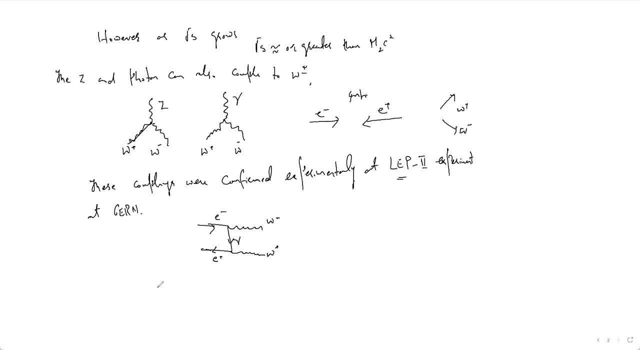 However, as I said, this Z and photon also have the coupling to W plus minus both Z as well as a photon. So let me represent these two diagrams with the help of a Feynman diagram, when I will consider this electron and positron into the consideration. 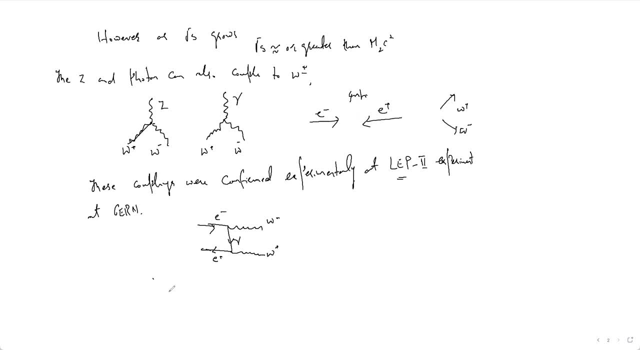 So what is actually happening? so let me represent it with the help of this Feynman diagram. So here we have, this as an electron, Let me represent this as an electron and this here as a positron. So there will be a some photon exchange and it could result in the production of a W plus. 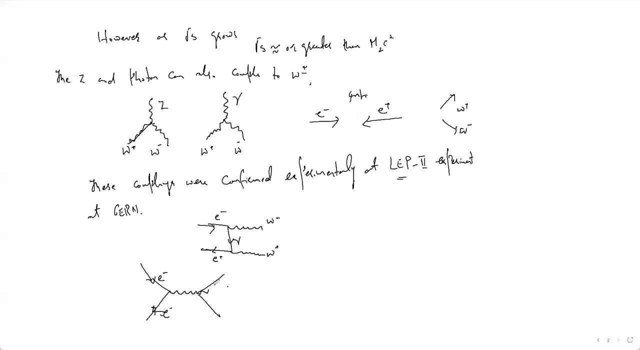 minus. So I am going to represent, because they are Gauss bosons, so I am going to represent it by this, not by the straight lines. okay, So this is W minus and this is W plus and, as a result, we here have a photon. So this, if you see this thing- so I was telling you- this photon will couple to W plus minus. 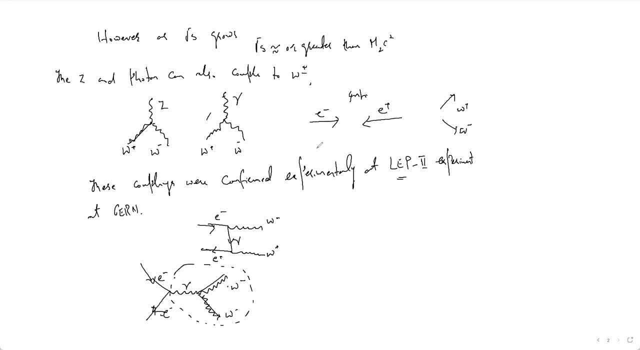 but photon will come out of something. so this photon actually comes out from this electron positron interaction, Hmm, As electron positron. So Grahame stopped perhaps in a whether in an electron positron, but which you can observe in não. we have really excavated electron positron, actually excavated to surreaction energies. 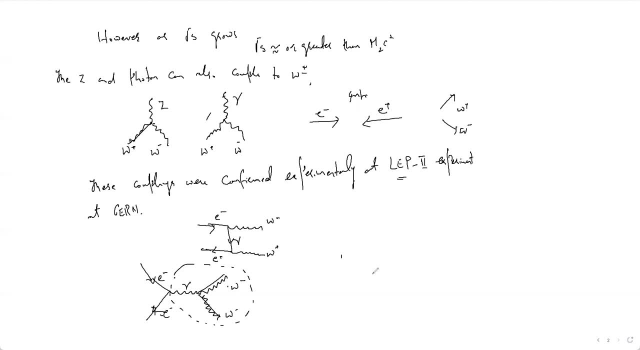 Also, what about this other process, the Breaking Elector spike algorithm? Exactly, what about this other process? we have this electron coming in and also we have a positron coming in- electron positron- and as the result, there will be a Z zero, which will then decay to. 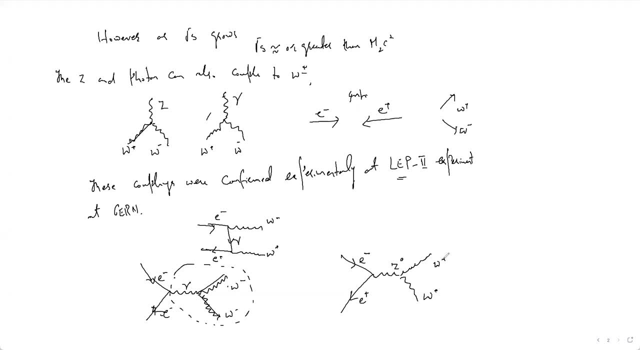 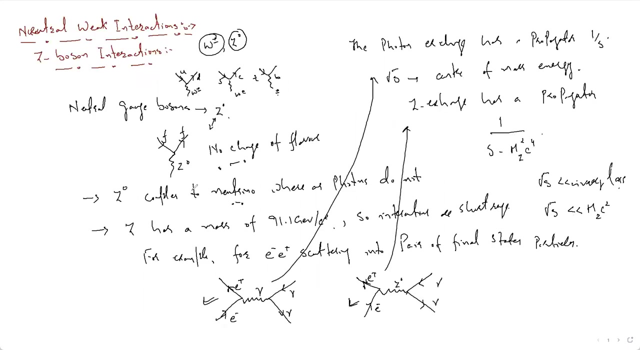 Go to some W minus and W plus, W minus and W plus. Okay, So this is actually happening in this weak interaction. So, okay, Now I will come to some another point, but I hope up to this point it's clear- I will just repeat the same thing. So, again, what I said after this particular step, I said, yeah, this neutral, weak interactions are actually caused by this exchange of this Z0 boson. 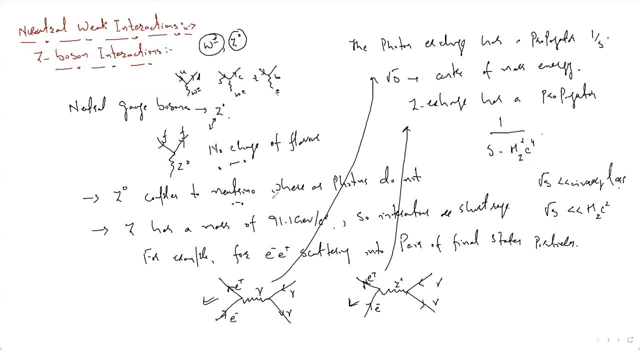 Okay, Then I see that these processes are similar to the photon exchange, but there will be certain differences. That is, Z0, this will copper to the neutron, whereas the Z and also the Z has a mass of this. Then I consider some electron-positron scattering, in which I said that the final pair of particles are being like, for example, electron-positron key. there will be an Z exchange, which will result in the production of two photons, and also the electron-positron. there will be an exchange of two similar, two processes. 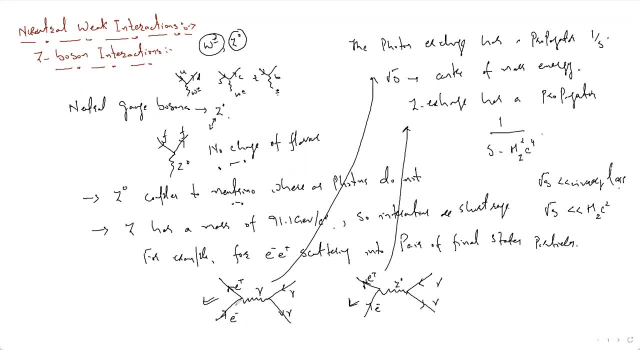 Then I say that both these processes have a different propagator. In the first case, where we have the photon exchange, it has a propagator of 1 by S, whereas this has a propagator of 1 by S minus Mz. 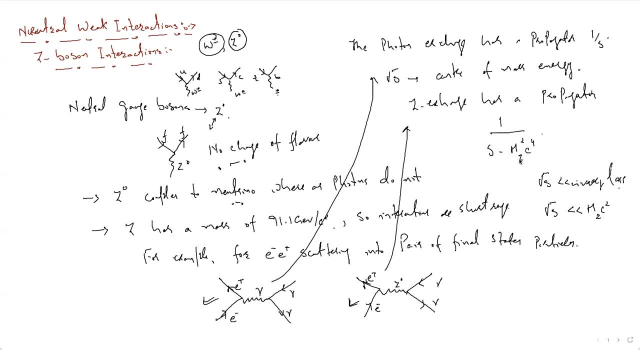 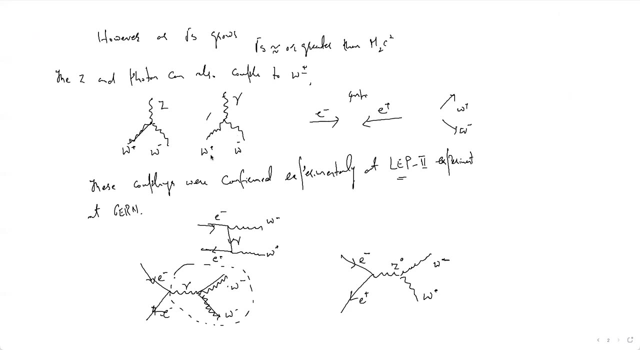 Then I do take different cases, when the center of mass energy is very low and when the center of mass energy is very high as compared to the rest of the bosons. Then I come to the other point. I say that this W plus minus, this Z0, and this photon and Z0 will also copper to W plus minus. 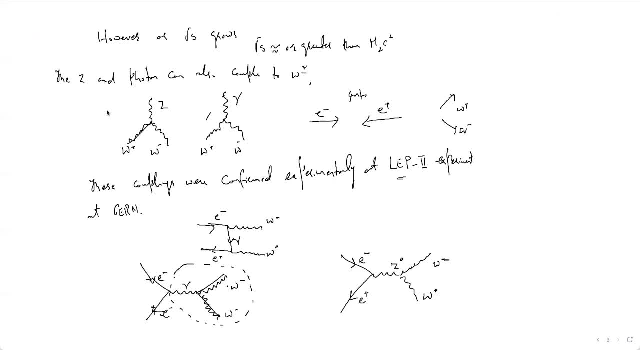 W plus minus, W plus and W minus, And these are actually confirmed experimentally at this particular experiment wherein the people actually accelerate this electron and the positron. as a result of when the electron will annihilate this electron and annihilate the positron, it will produce a photon which then decays to W plus and W minus. 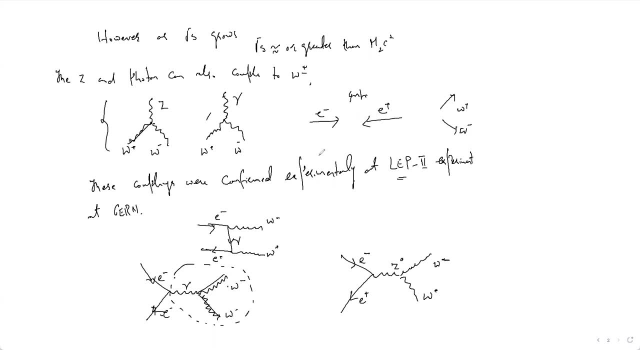 The energy will remain conserved in the process because they are being accelerated at very sufficient energies. okay, So these have some masses, some energy is being converted. This photon has enough energy that It will be equivalent to the energies of, Because the mass here will be taken into as an energy. 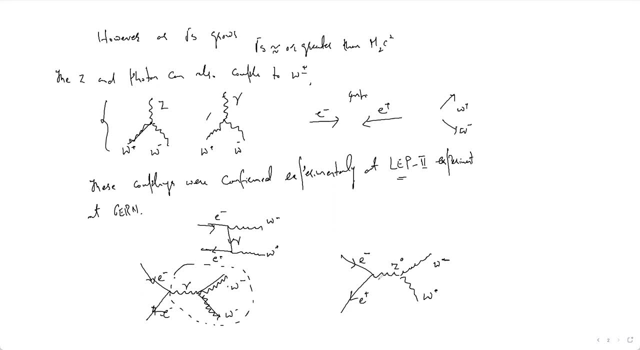 Similarly, I have this process also from that very experiment that this electron positron will annihilate. As a result, it will produce the Z0, which Z0, then, will decay to a W plus and W minus. right Now you might think W plus and W minus is actually having the 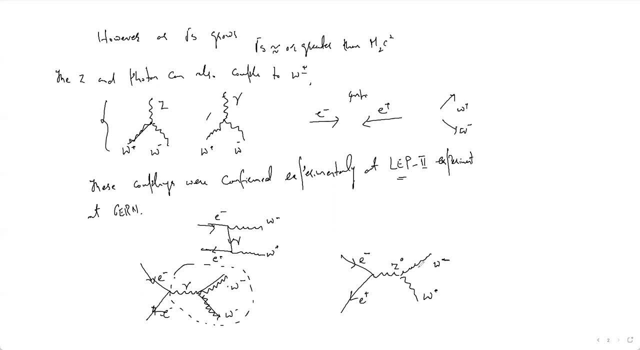 Their mass is more as compared to 41, and their mass is less. But because this Z0 has enough, It has enough energy and, as a result, the energy will be converted into the masses. energy will remain conserved in all these processes. okay, 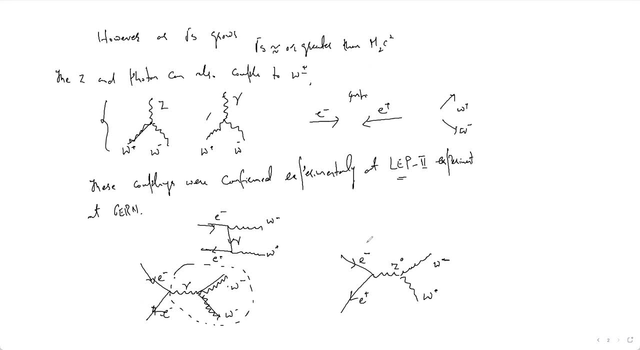 So the purpose here is to say that this Z will couple to W plus minus and also the photon will couple to W plus And if Z is converted into photon, W plus and W minus boson and also we can have Z0. 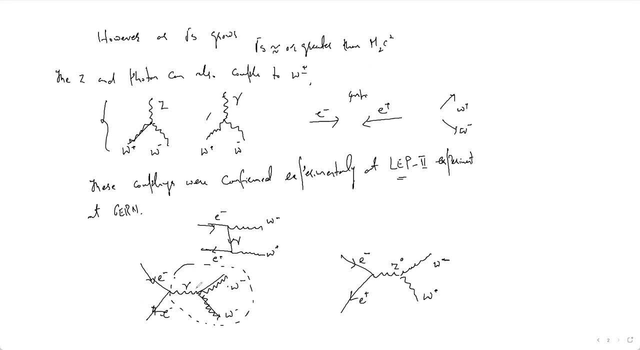 Now this is the fenomenal representation of both these processes, where we have the photon exchange and where we have the Z0 exchange And these. So This was actually predictive, theoretical, but later on these findings were confirmed at that particular experiment. 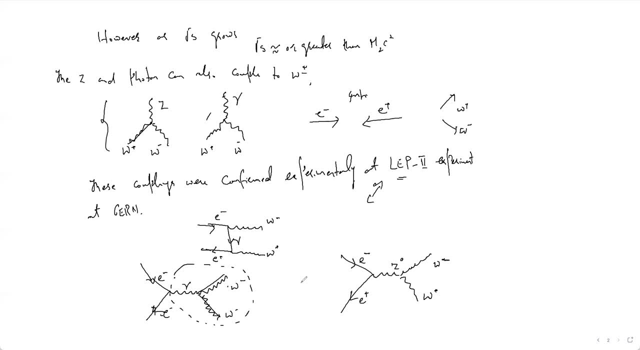 So we have strong experimental evidence of these processes- Yes, that these processes are really happening. Okay, Let me now come to another point. So you might have known about the electroweak theory. I don't know if you know about this or not. 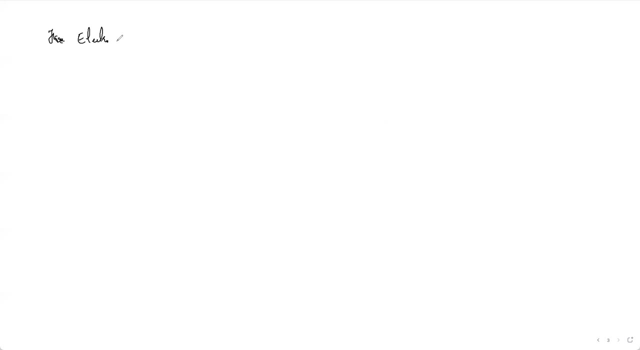 Electroweak theory. Electroweak theory is that Electroweak In electroweak theory, since you know that we have four fundamental forces: one is strong, then there is weak, then there is electromagnetic and then there is gravitational, and the people are working on the unification of all these forces. 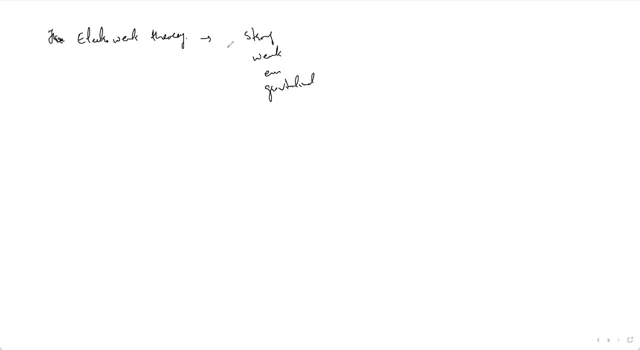 Unification means we are going. People are actually trying to see that all these forces are the manifestation of one single force, which is called grand unification, Grand unification, Okay, So people have not. People have not actually achieved up to that point, because the gravitational force is creating some problem. 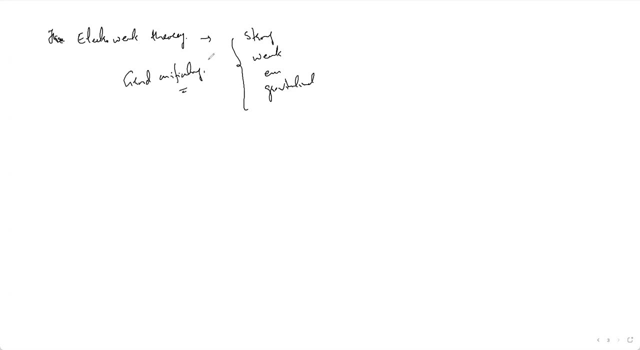 That is some different issue. different topic, that is electroweak theory. But here I mean to say, since you know, that earlier the electricity and the magnetism were considered as two different forces, but later on, with the help of a Maxwell equation, we see that this electric and the magnetic, they are actually the manifestants of one single force. that is what we call as an electromagnetic force. 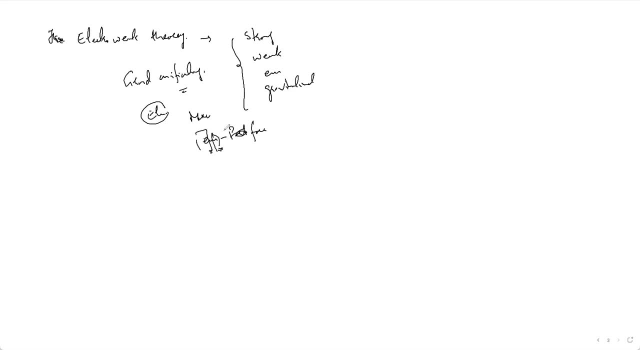 This is electric and the magnetic oscillations coupled together. So this actually Now, later on now, since the electromagnetic and the weak, so there were the people who actually so, when electromagnetic force and plus the weak force, so we are actually saying that these two forces are actually the manifestants of one single force. that is what we call as this electroweak force. 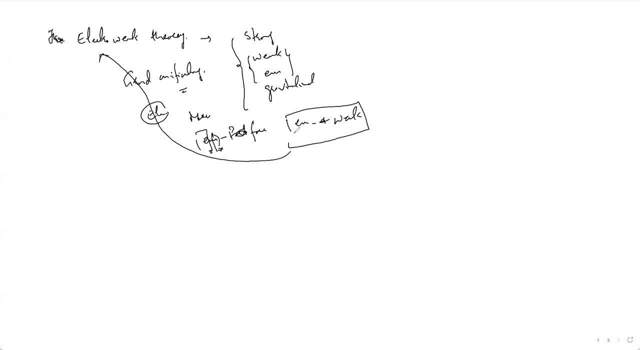 So it actually contains electromagnetic field as well as the weak force. So this theory was actually proposed by a few people, and maybe I don't know whether you know the name of those people or not. One of them is very, Very known to us because he belongs to this region. 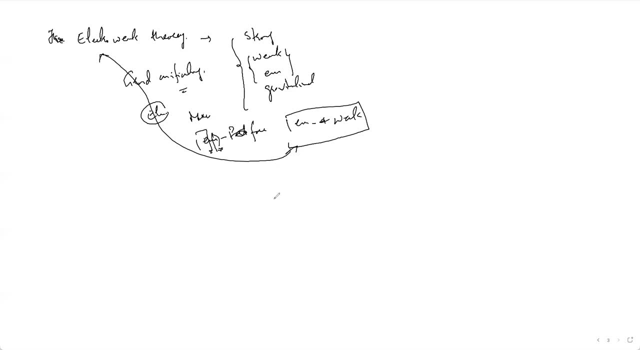 The region means he was from Pakistan. So there were three people actually. One is Glyasau, Another was Weinberg, And then there is Salam. Salam is This is called Professor of the Salam. Actually he was from Pakistan. Right now. after that, he was exiled for certain reasons. I am not going into those details. He was exiled from Pakistan. He resides there in Italy. If you look at the ICTP, there is an ITCP International Theoretical. 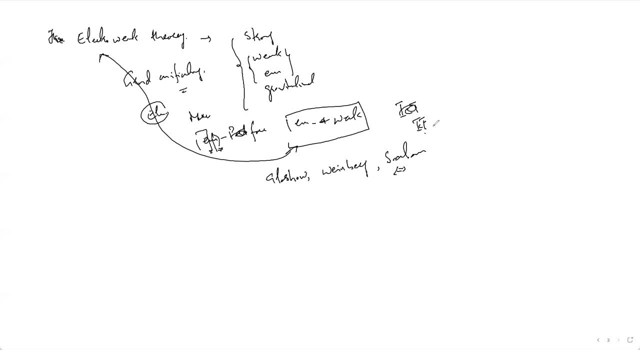 ICTP or ITCP, something like that- International Theoretical for International. ICTP, International Center for Theoretical Physics, ICTP- International Center for Theoretical Physics. That is a very reputed institute in Italy. Actually, it was he who actually 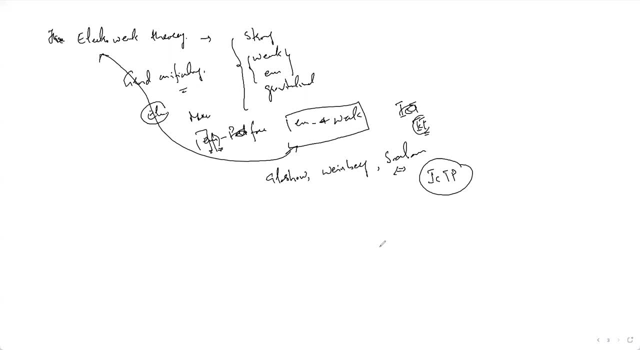 Hmm, Hmm, Hmm. Who actually started this ICTP? Professor of the Salam. Okay Now, so This is actually a different thing. unification of the forces or grand unification, That is actually a different topic. But here, since we were discussing the weak force, so I will just tell you. 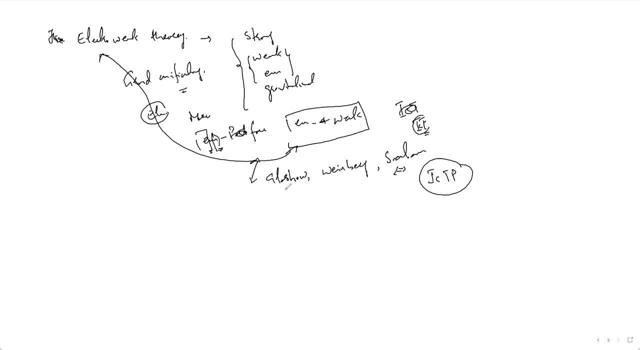 So this electroweak theory was actually developed by these three people, Glyasau, Weinberg and Salam. So that gives actually the relation between the weak coupling They actually. So one is Glyasau. They actually gave this to the electroweak theory. they gave it in terms of some. 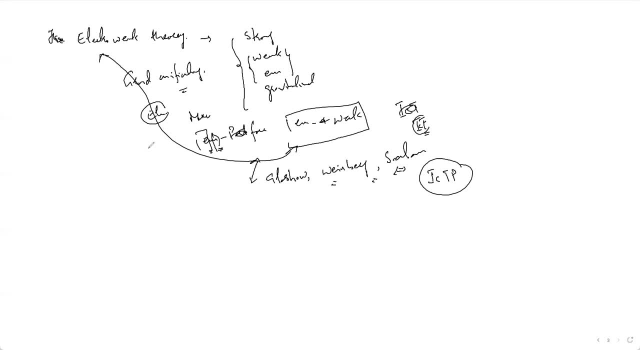 This What we call as a formalism. So you know that then we have, Like in the previous case I told you, GW for their current, current interaction, And we showed you how this GW depends upon what the things So, this electroweak theory. they give the relation between the weak coupling, relation between the weak coupling and the magnitude of electric charge, E and the mass of Z and W. 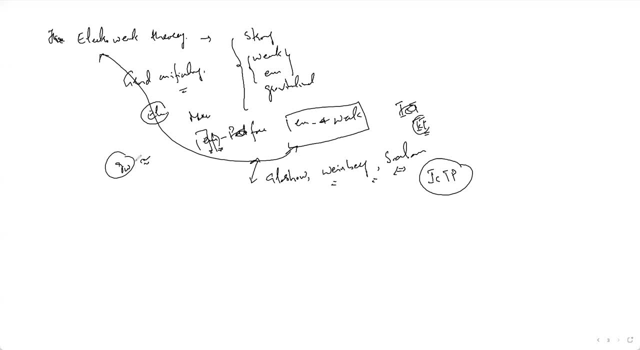 W plus m, w plus minus. so they so developing this electroweak theory, they obtain the relation between this gw, then we have the magnitude of electric charge, e, then the mass of z and mass of z and mass of this w plus minus. in terms of all these things they give this coupling okay. so what? what? 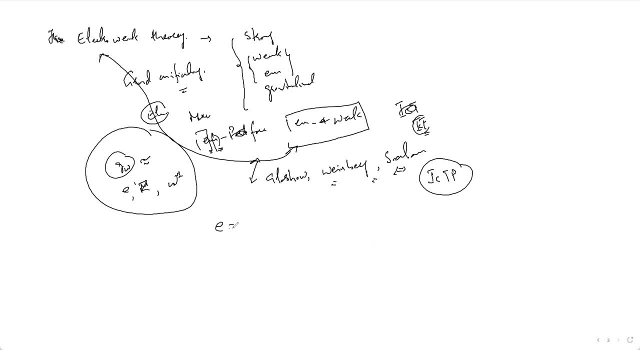 is that relation? so the relation is like this: charge e is always given by in terms of weak, this coupling, gw, sine of theta w. okay, this is a relation. so we have, uh, this weak coupling constant. now you will see so. so it just weak coupling will involve the mass of z as well as 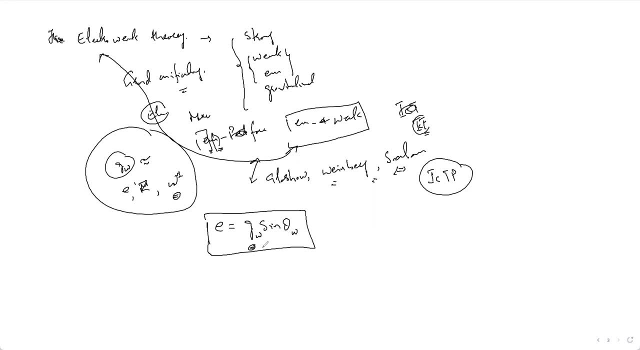 the mass of w plus, minus and sine of theta w, now theta w. what is theta w here? theta w is called, as is known as, weak mixing angle. weak mixing angle- okay, you, this is known as a weak mixing angle and this is given by something we are going to discuss. 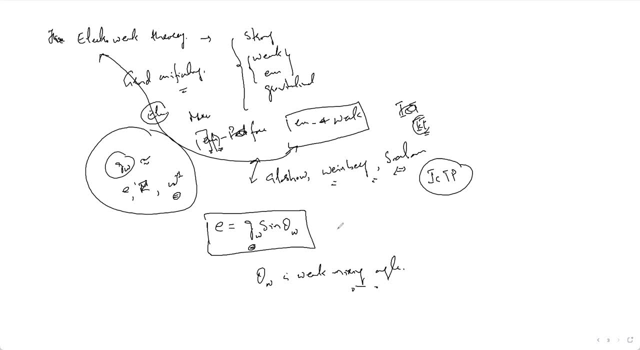 this weak mixing angle in the next lecture, which is the what we call as a cabibbo theory. so we are going to discuss it in detail there. so here this is: gives you actually the relation between the electric charge e, the weak coupling constant q and also the masses of the w and w. 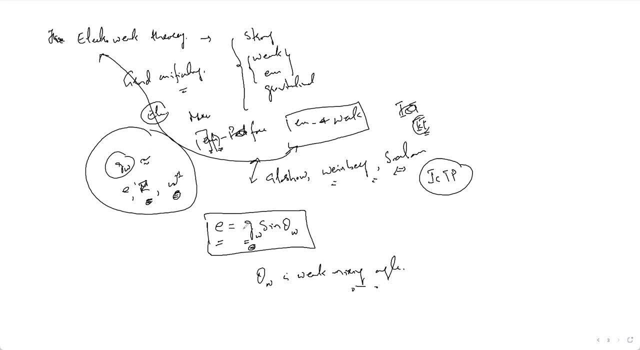 plus minus. okay, there is a very complex mathematics behind this particular this equation, but we are not going to into that detail, so i'm just taking you directly to this particular equation which will give you the relation between this electric charge, e because this? because, as i said, this is an electroweak theory, so it will involve both. 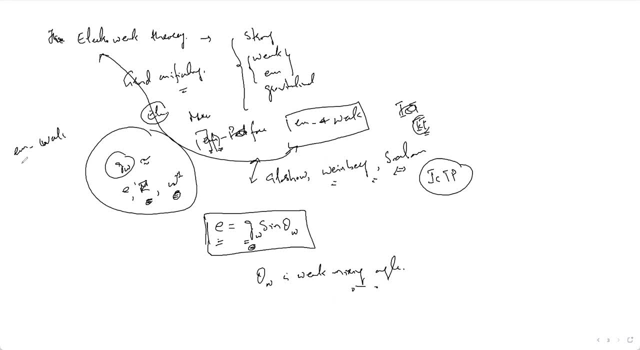 electromagnetic as well as the weak force. so this charge will come from the electromagnetic part and a week. you know that this is we. the g w is the weak coupling constant and sine theta. sine theta is some weak mixing angle. now how this speaking mixing angle is defined as this weak? 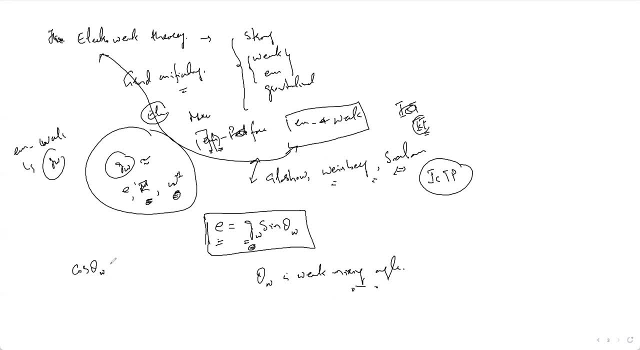 mixing angle is always given by some cost of theta w is equal to m, w is equal to delta w. we are not requiring this kind of怎麼 to use this weak mixing angle and this is an even difference between. we keep calculating this. we keep calculating at least the least possible and, as you'll, 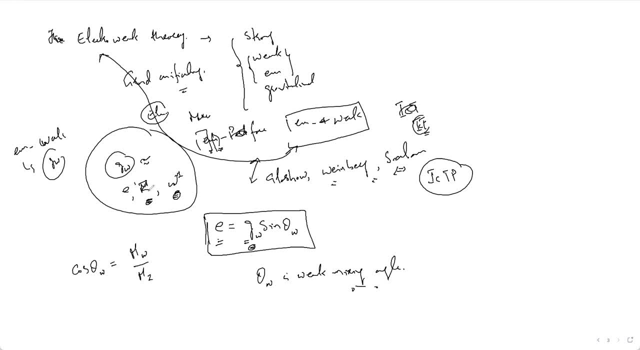 by m, z. okay, so this is why these two particles actually are taking taking their role. one is z zero and up. so we actually define this weak mixing angle cosine of the theta w and it is given by mass of w plus, minus and mass of z zero. obviously you know that. what is the mass of w? 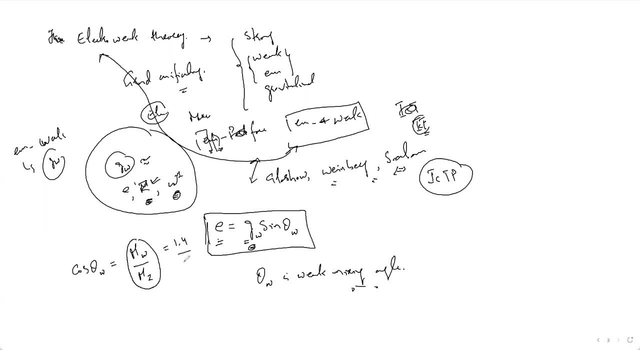 that is some around some 1.4 or something, and this is around some. what is it 144? so 144 or 142 divided by this 91, so obviously there will be some value to this corresponding we are going to discuss and that is called cabibor angle. just combat me, okay. so this theta mixing angle is: 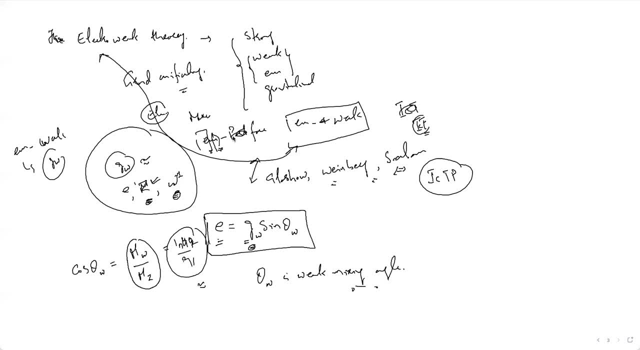 given in terms of a mass of w plus and mass of z zero boson. okay, so well, in that case, how we can also represent. now you know that from this very elementary level, from the elementary classes, you know that sine theta is always given by 1 minus cos square theta, sine square theta, right or i? 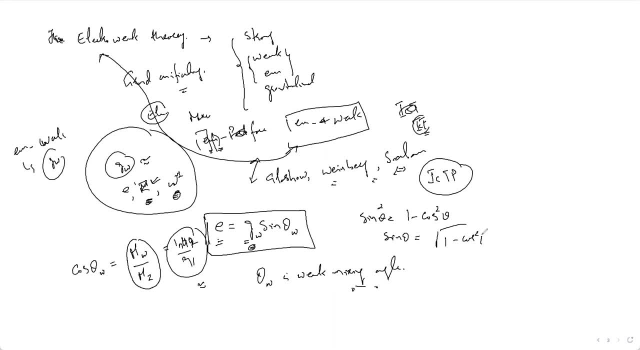 can say that the sine theta is under root of 1 minus cos square theta. okay, so, using this particular relation, you can see that this. i will write down this energy in terms of this weak mixing angle. so you can write down this particular equation: as this e is given by g, w, then under root of, because. 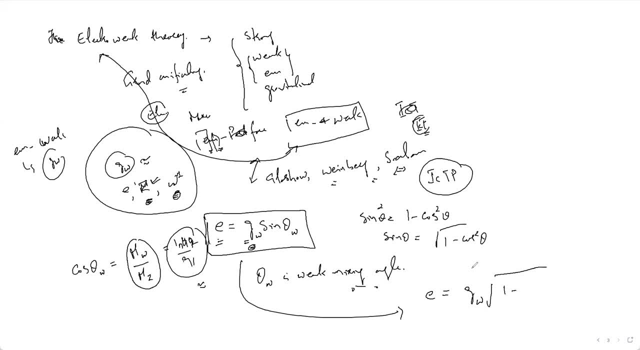 sine of theta w, it will be 1 minus cos square theta w. so 1 minus cos square theta w, that is m w square by m z square. okay, so using this, we have the weak coupling condition we have. we know the. we have the mass. we can find out the relation between all these things. right, okay, now add. 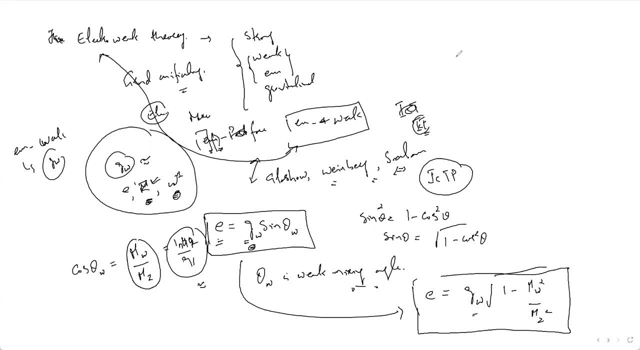 energies maybe less than m w c square. okay, okay, now add energies. add energies very much less than m w c square. anyway, when we have the energy very much less than m w c square, m w c square is around some 141 gv, so that means when the energy is very much less than this one. 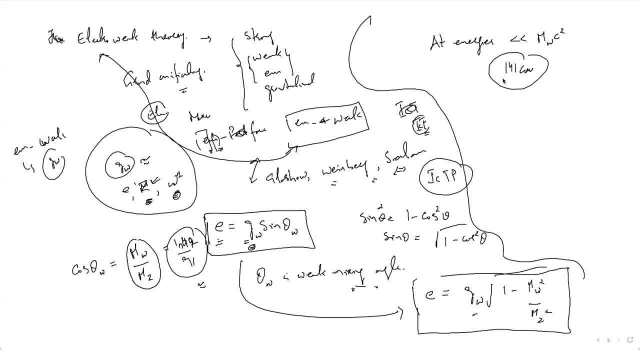 141 gv. the amplitude of this w plus minus exchange, amplitude of this w plus minus exchange process is proportional to. is proportional to what is it? that is the amplitude of w plus minus exchange. that is the probability of this w plus minus section. it will be always proportional to. 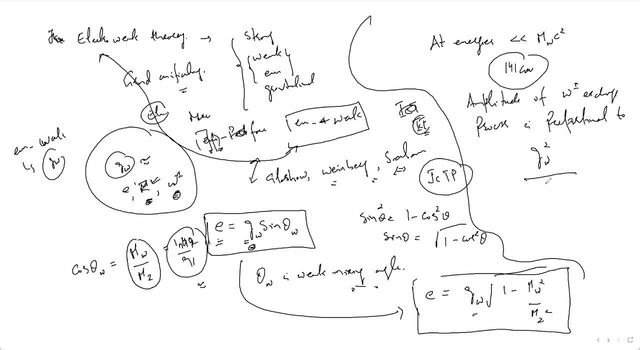 and it will depend upon this: g w square divided by 4 pi epsilon naught 4, pi epsilon naught m w square, c: 4. okay, so this is the amplitude of the amplitude of w plus minus. exchange is processed by given. so we know that we coupling constant, we know this. this is a cone standard again.